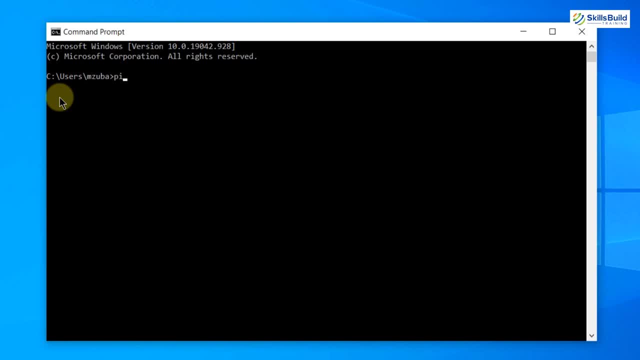 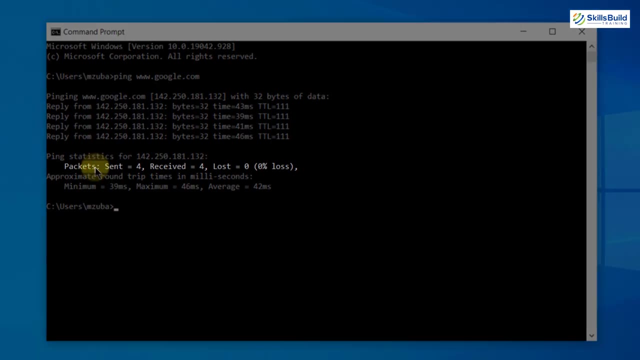 and not from the internet service provider. so just write ping and after that I will write wwwgooglecom. just hit enter and here you can see we have sent 4 packets and we got 4 packets back. as you can see here, it says packet sent equal to 4, received equal to 4 and because of that our lost is 0. so this is. 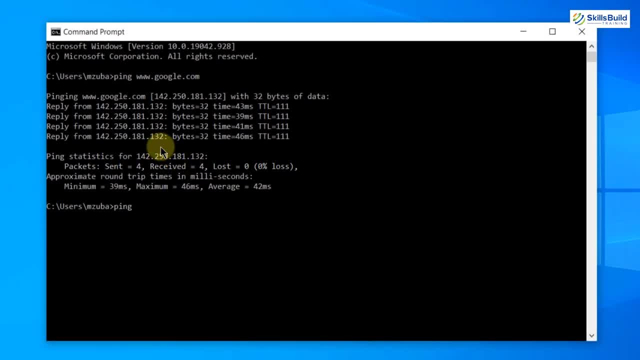 how ping command works. let's have another example. so this time I will write an ip address. so i will write here: 192.168.2.200. just hit enter and here you can see it says: request timed out mean we are not been able to send our echo message to our destination. 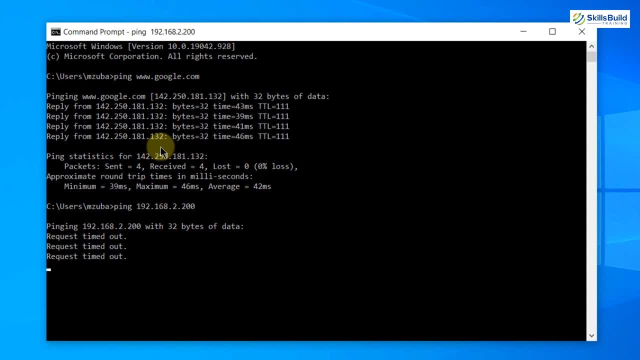 and that shows that our destination is not reachable or you can say it is not available at the time. so this is how we can get to know that if the destination or a particular ip address or a particular network is available or not. so this was all about ping command. so i will clear my. 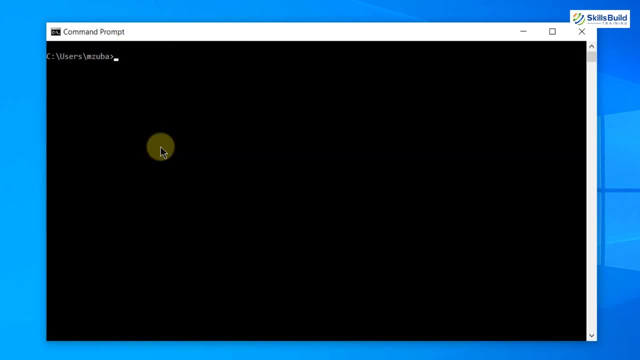 command prompt here for that. just write cls and hit enter number two, ipconfig. well, the ipconfig command displays all the current tcp and ip networks configuration values and along with that it also gives you the basic information to get your ip address, dns server ip address, your router's ip. 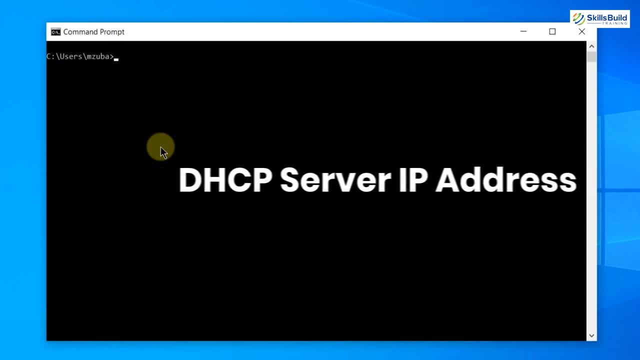 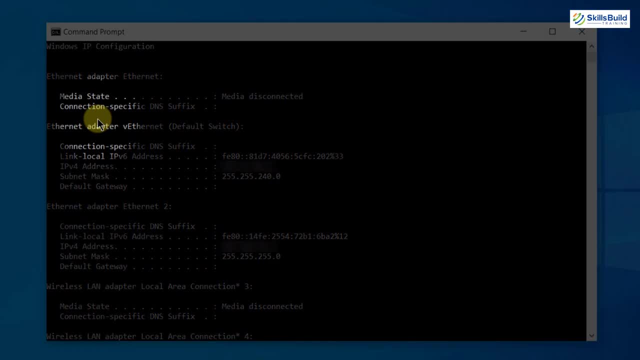 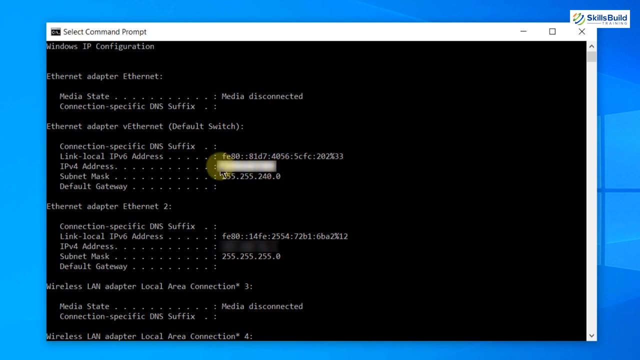 address and dhcp server ip address, etc. so now i will write ipconfig here. just hit enter and this is my network at the moment. here you can see that we have ipv4 address. means this is my ip address. means if someone want to connect to me or someone wants to communicate with me, they need to use my. 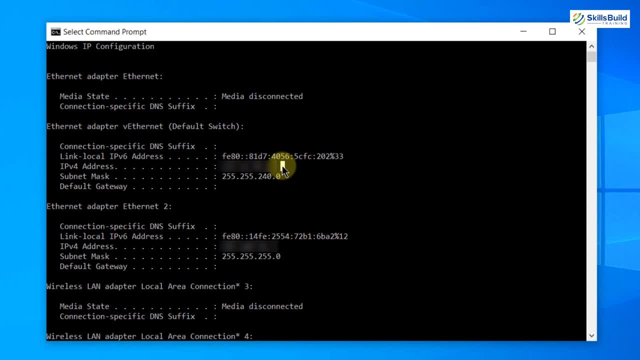 ip address and my ip address is this one, and down here we have subnet mask and down here we have our default gateway. at the moment, computer uses ipv4 address means if someone want to communicate with me, they have to use this ipv4 address of mine and they also need my subnet mask to reach. 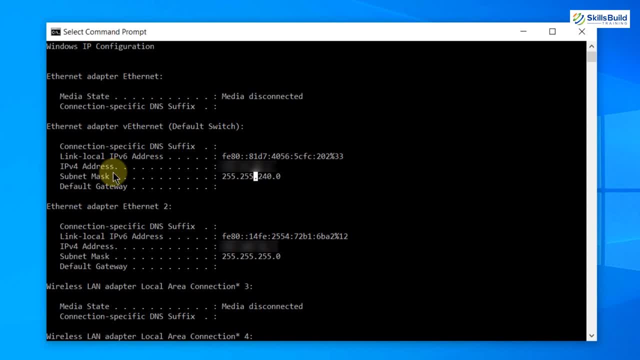 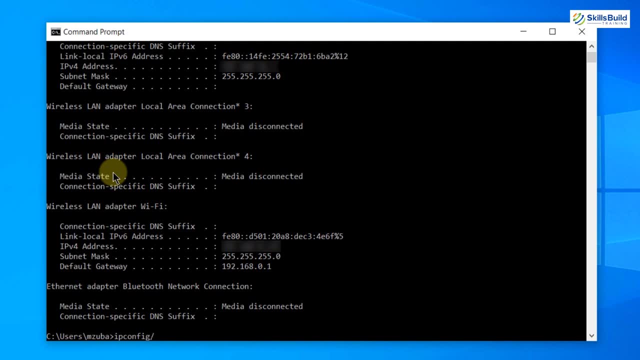 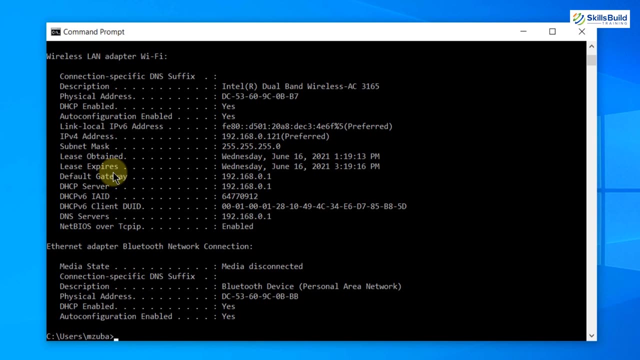 my destination. so that was all about ipconfig number three, ipconfig slash, all. so i will write ipconfig slash all, hit enter, and here you can see that we have more detailed information about the dhcp server. and then we have our dns server here as well. one thing is very noticeable here. my 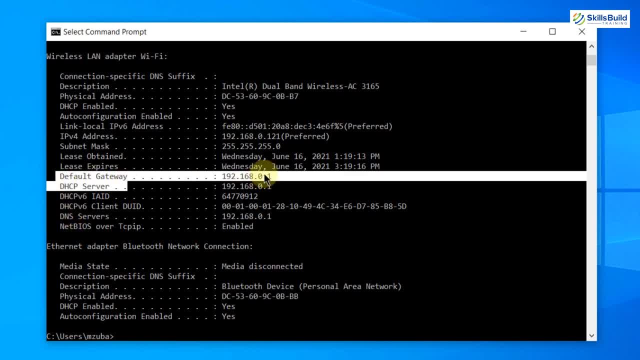 default gateway is this one, that is 192.168.0.1. it means this is my router. default gateway is always your router. but if you come down at the dhcp server and here you will notice that it has the same address as my router, and here you can see that it has the same address as my router. and 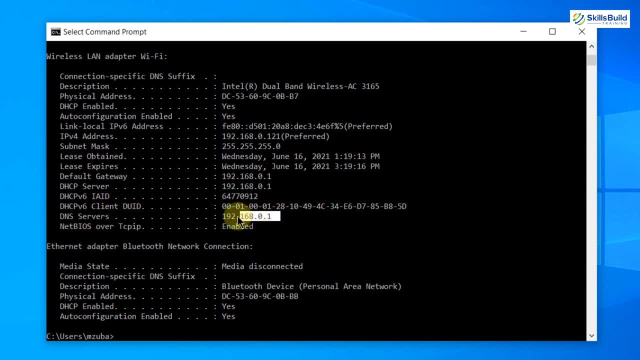 if you go down in dns server, it has also the same address as above too. it means that my dns server and my dhcp server, they both lies on my router, and if i want to do some tweaks, or with my dhcp or my dns server, i can do that from accessing my router. so this is how this command ipconfig- slash all. 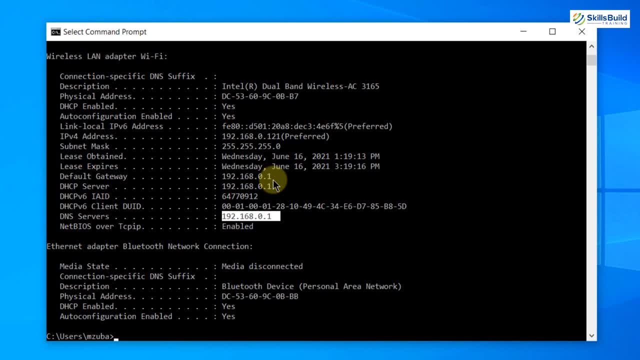 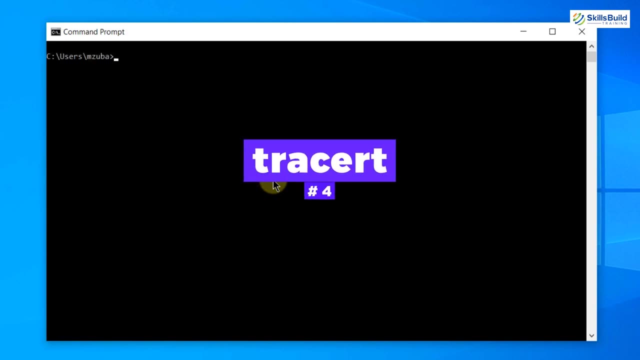 is helpful as it gives you the information for the troubleshooting for the network, and obviously for troubleshooting you need information, and ipconfig slash all has all the related information which you need. i will clear my screen. first, number four, tracer t. this command helps you to see the route. 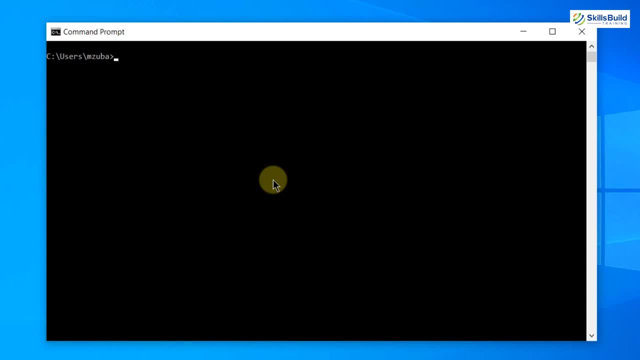 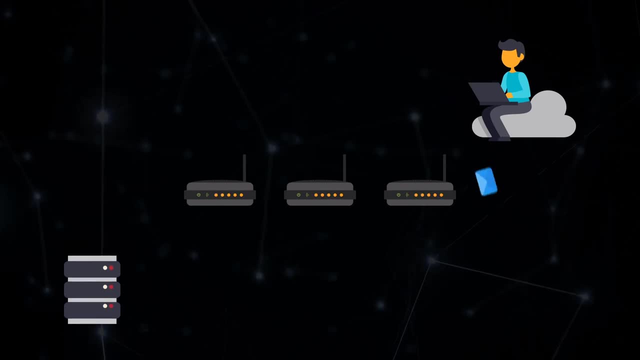 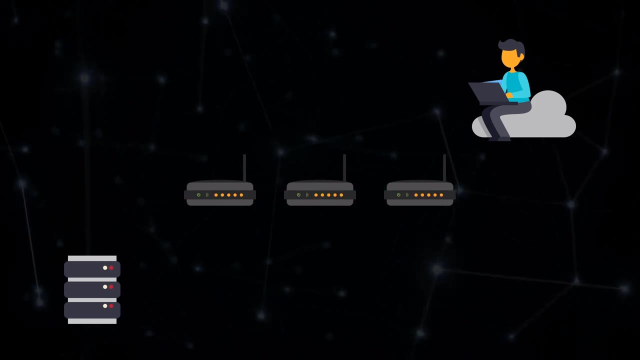 in step-by-step format. a packet has taken to go from host to the destination which you have specified for it. for example, if you send a packet to google or some other destination, the packet will not go to google directly. instead, it will go through many different routers before finally it reaches the googlecom. so i will write. 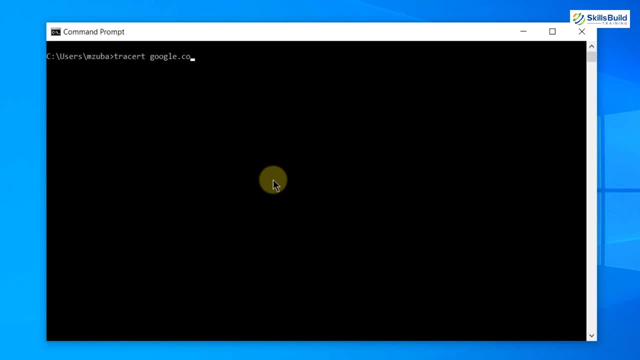 here: tracer t, googlecom, hit enter and here you will have all the information that from where my packet got started and then how it reached to the googlecom, my packet has started from router and then it went to this router, which is neotelpk, and after that it has moved toward the third router. 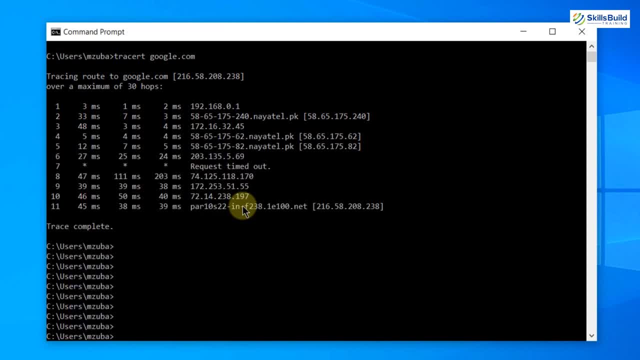 and in the same order it will reach to the googlecom. and here we are done with our trace. and my packet has taken 11 routers in total and one router was not responding. as it says, request timed out. so this is the information about the path the packet has taken from host to the destination. so i will clear my screen. number five: 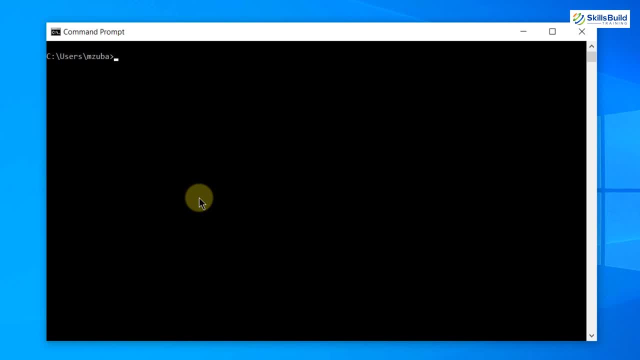 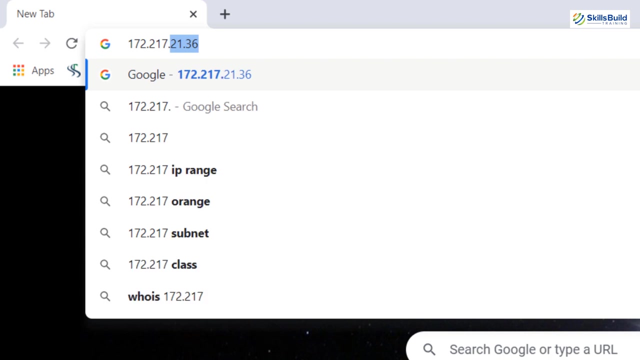 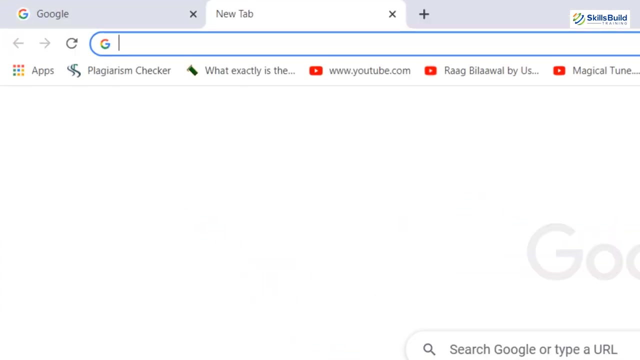 nslookup. by using this command, we will be able to fetch the dns records for a given domain name or the ip address for those who do not know. ip address is the mathematical form of address of any website. for example, let me go to my browser here. if i write 172.217.21.36 and hit enter, it has taken me to googlecom, and same as if i write: 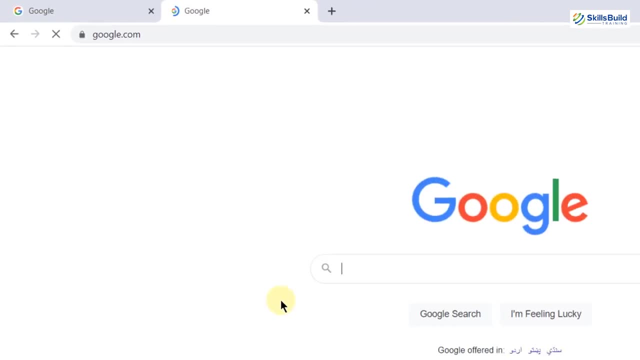 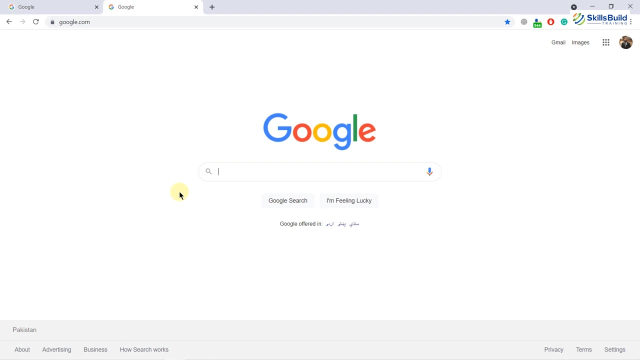 googlecom. it will take me to the same destination. so ip addresses are the mathematical forms of address of any website, because it is not easy to remember the ip addresses as they are in numbers. so the ip addresses and the domain names are stored in a dns server, which means dns server. 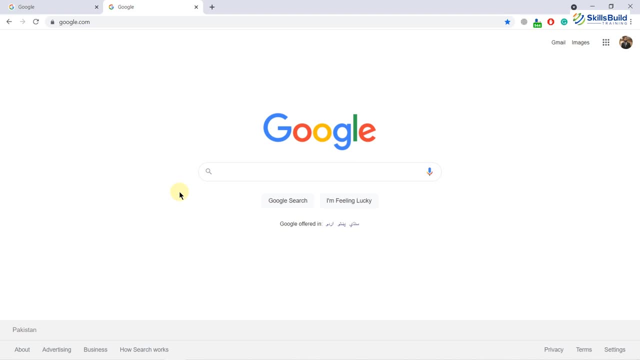 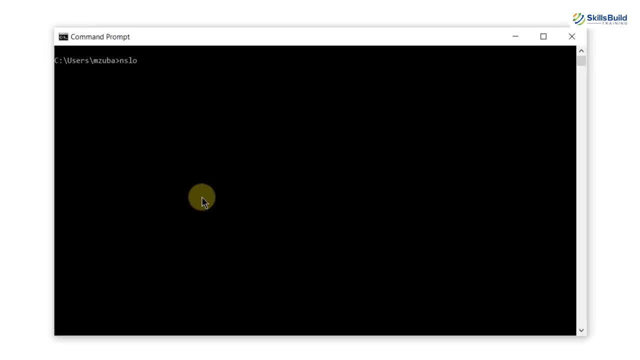 is responsible for all this. with the help of nslookup command, we can query the information about the dns records. so here i will write ns, lookup space, googlecom, and hit enter. so this command has given me this address. so if i copy this address and now if i go to my browser and 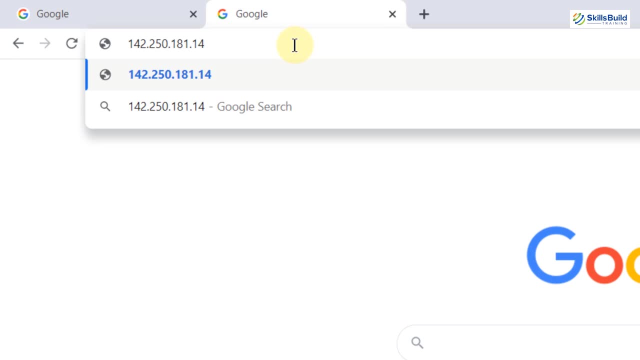 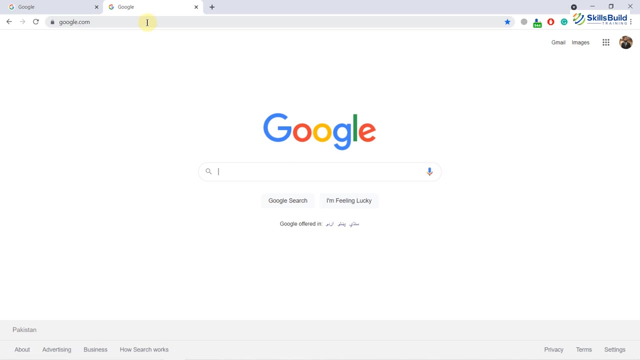 paste this address which i got from using this command: hit enter. now it has again taken me to the googlecom. so what this command has done? it has given me all the ip addresses associated with an address. it means google have almost 10 to 11 ip addresses, which gets used to reach the google. 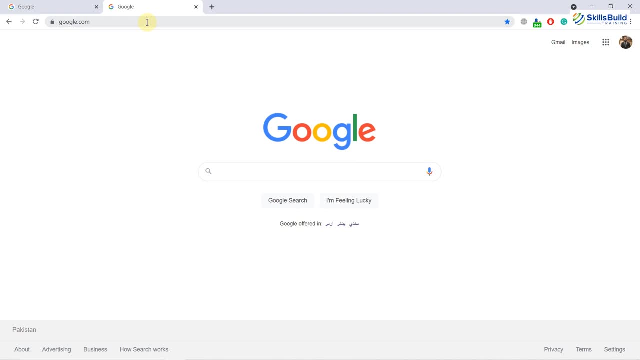 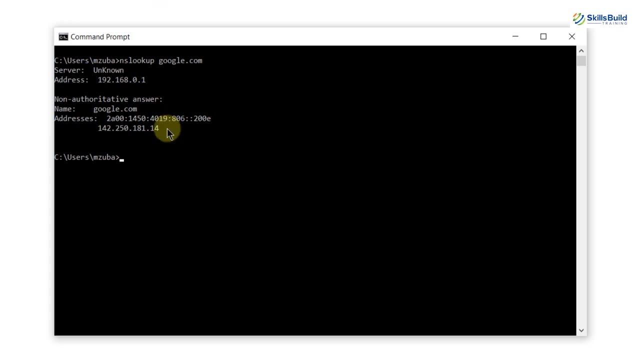 so, if you remember, earlier i used 172.8, 217.21.36 and now this nslookup command has given me a different address. so what this command does? this command gives the ip addresses of any website or any web page you want to see. i will clear my. 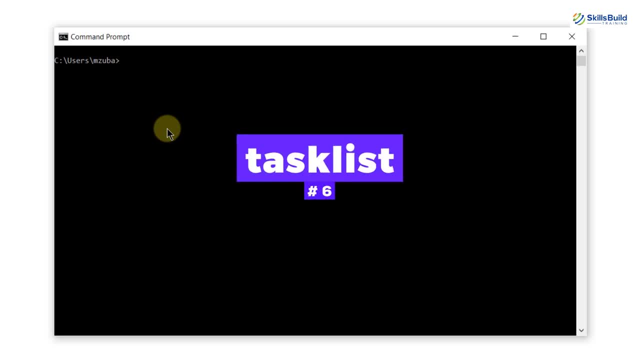 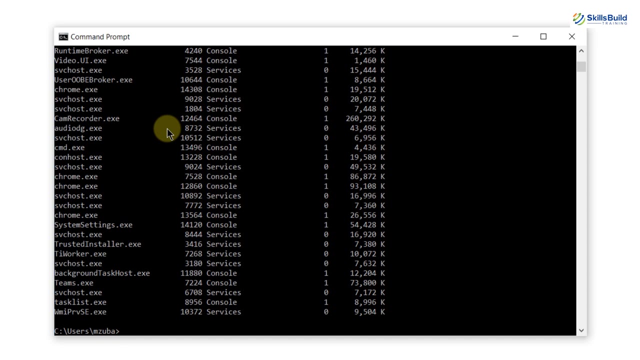 screen. and now let's move ahead, number six, task list. well, task list allows you to see for the tasks which are running at the moment in the system. so i will write here task list, hit enter. these are the tasks which are running at the moment. in many cases our system gets stuck and 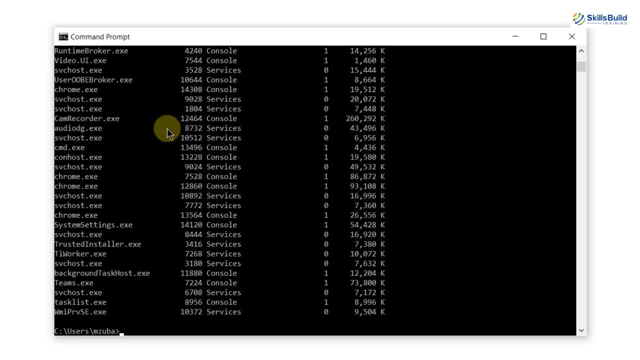 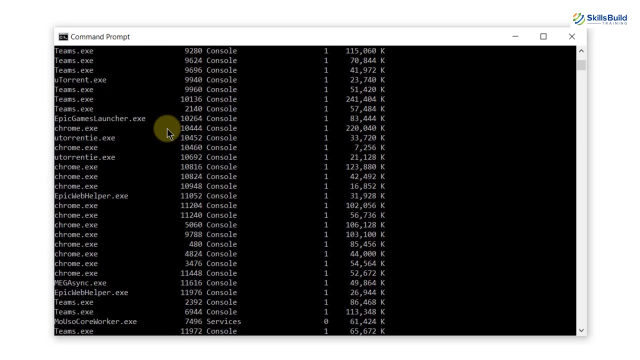 this is because we have lot of tasks running at the background. what we can do: we can terminate some of the tasks to make our system work perfectly again. for that we will use task kill command. so, as you can see, we have these tasks available or running at the moment. what i can do: i can remove. 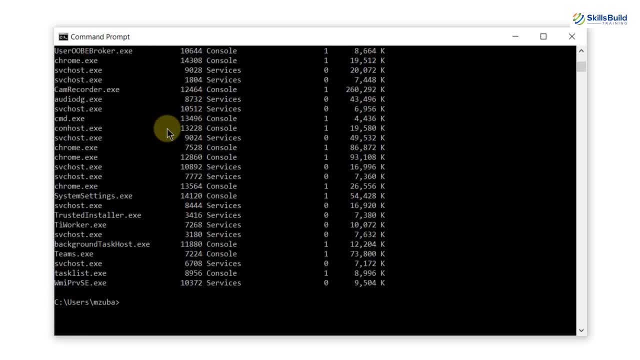 any of these tasks. for that i need to just write task, task kill- space backslash im. so here i need to write the task which i want to terminate, so let's terminate the cmdexe. this is right here, so i will write cmdexe- space backslash capital f. 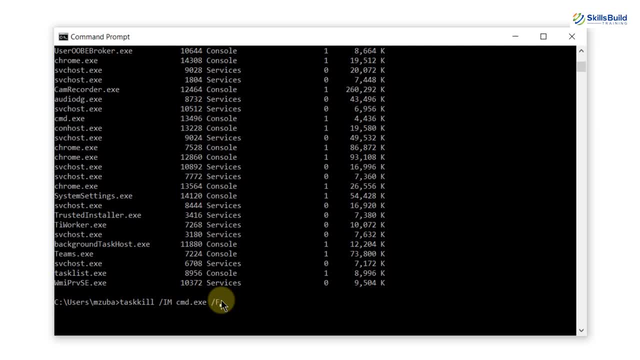 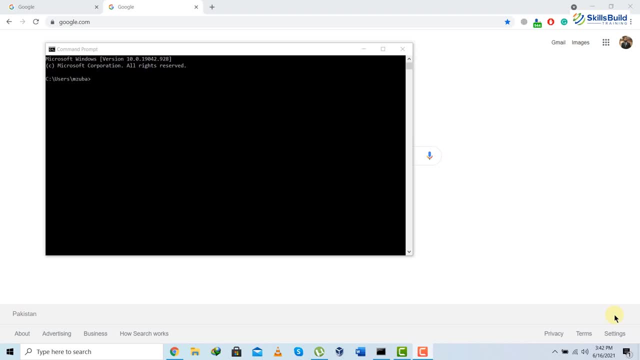 now, if i hit enter, my command prompt will get closed, and here you can see that it has just killed the task number seven: net sh. net sh is another very powerful command allowing you to view and configure almost all of the network adapters in your device in much greater detail. 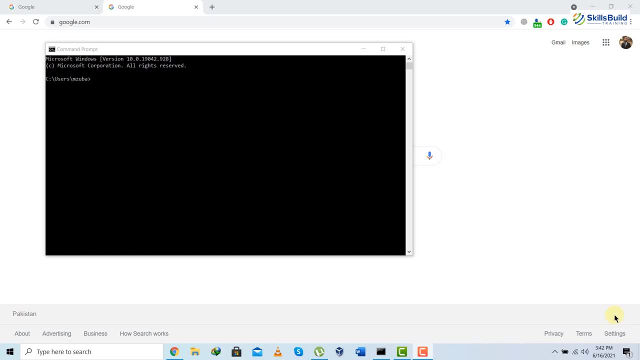 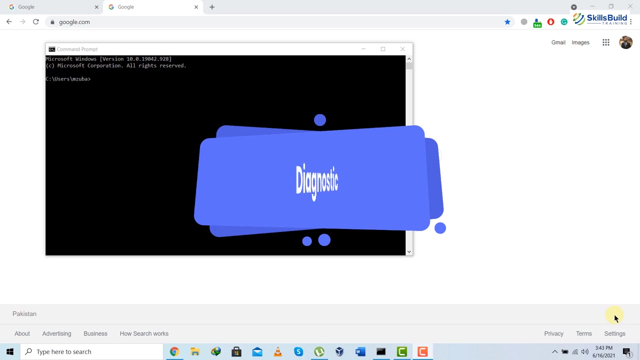 compared with some other commands available. when you run net sh command on its own, the command prompt will be shifted into network shell mode. within this mode, there are several different contexts, such as we have a context for dhcp related commands, we also have a context related to diagnostic and we also have one for routing. it is still possible to run individual commands. 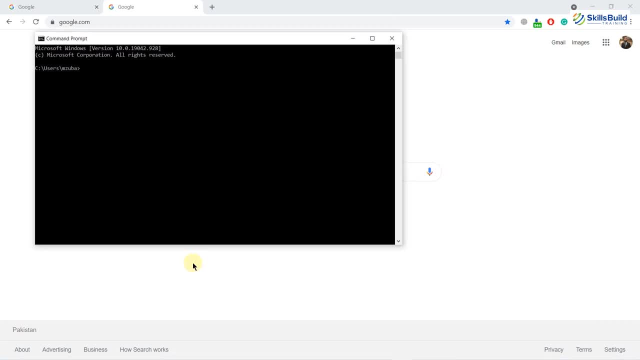 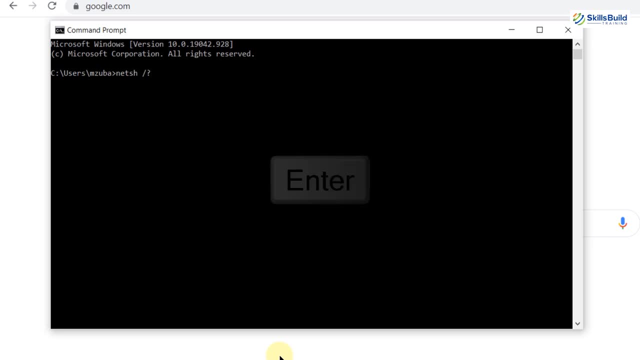 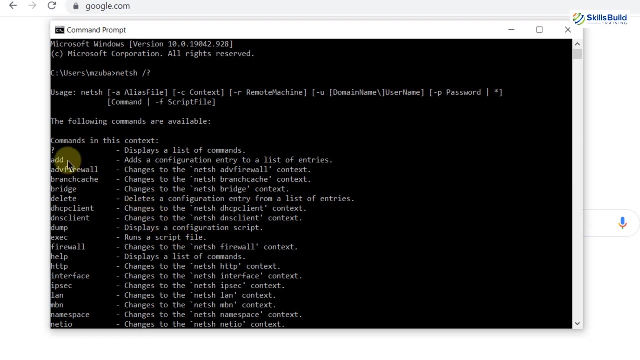 from net sh. so in order to see that what commands are available within that sh context, we just need to write net sh, space backslash question mark and hit enter. so these are different commands which are available related to net sh, so we can use any of these commands. so 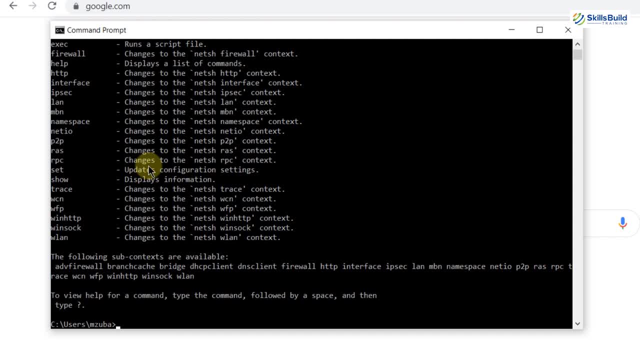 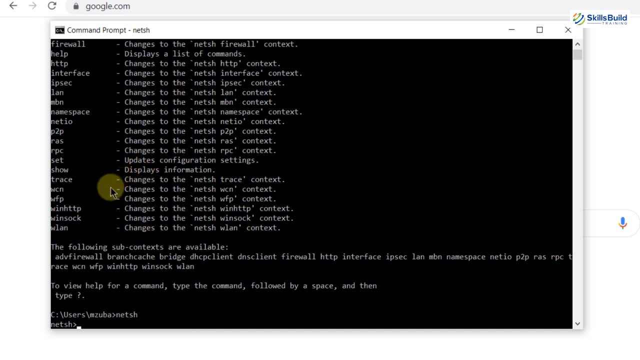 this is the command and this is the context. so what i need to do now i just need to write net sh, hit enter, so we are into shell mode. so here i can write any command for different contacts and i'll be able to get the information and i'll be able to do a lot of things. so we are done. 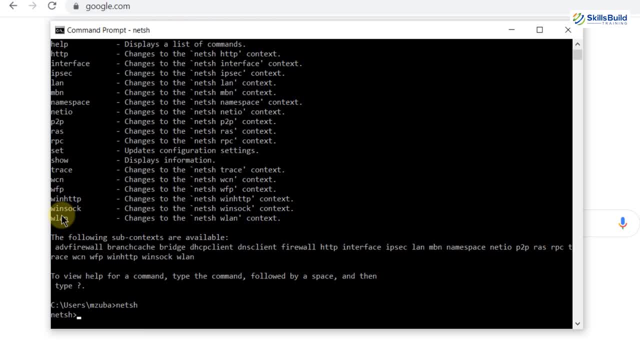 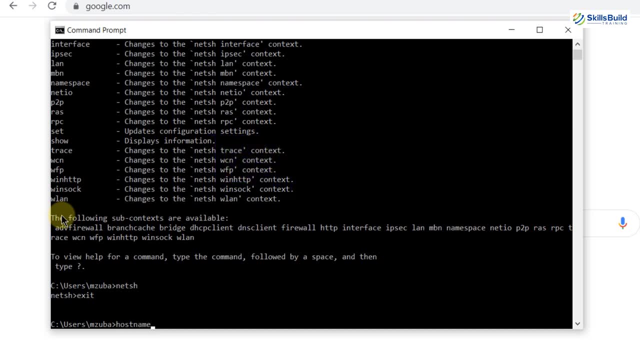 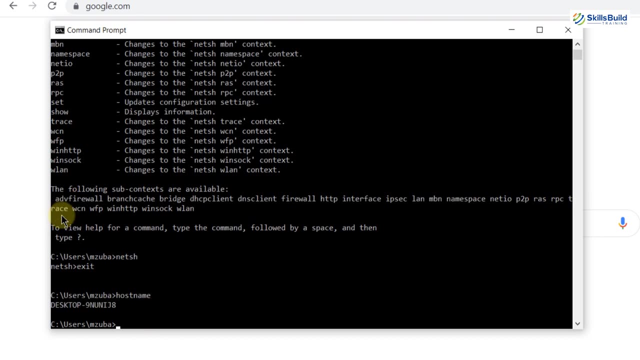 with our seven commands. now let's have some bonus tips, so let me exit my shell here now. first one is host name. i will just write host name here and hit enter. what it will do? it will give the host name which have been set for my laptop. i will hit enter and here it. 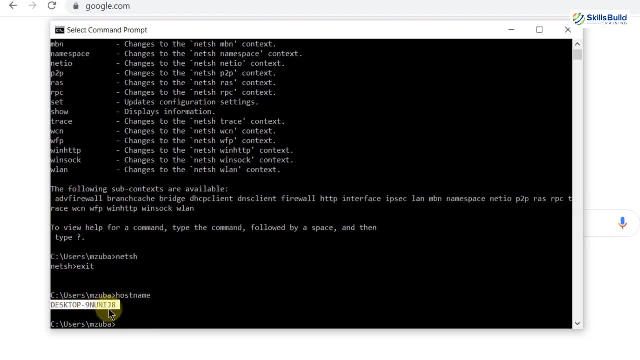 is my host name? is this one? so this is how easy it is to find out about host name. so if you have everywhere host name- i meanpl armor over services or devices- it will give you the address and now you do not have to go to your settings and then system and then. 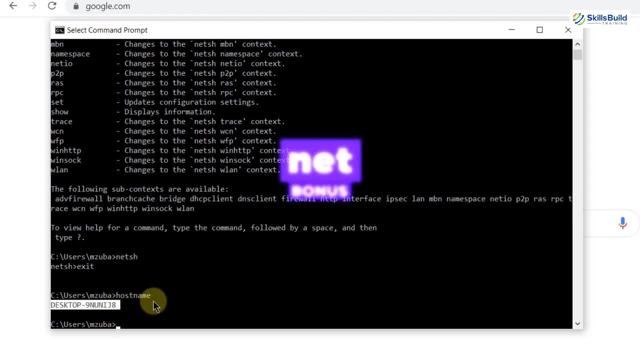 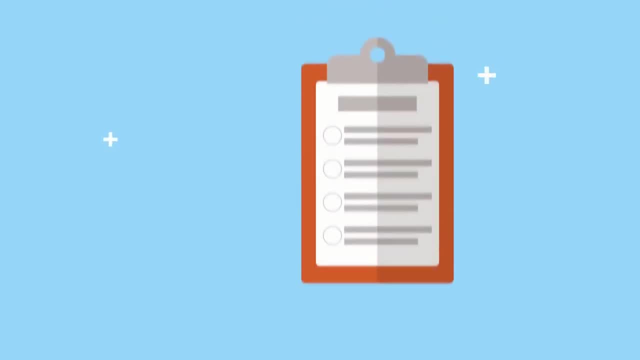 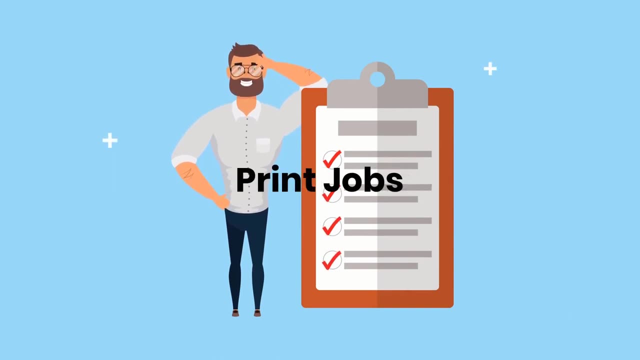 there, look for your host name. next bonus tip is net. well, it is used for displaying available NET switches. the net command is definitely a versatile one, and it allows you to manage many different aspects of our network and its settings, such as network share, print jobs, users and a lot more things. running just net won't do much, so what i will do now? 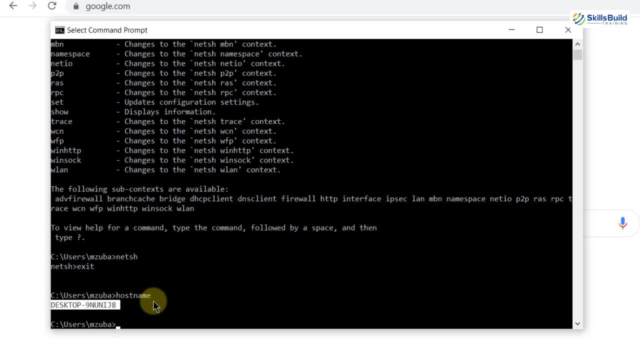 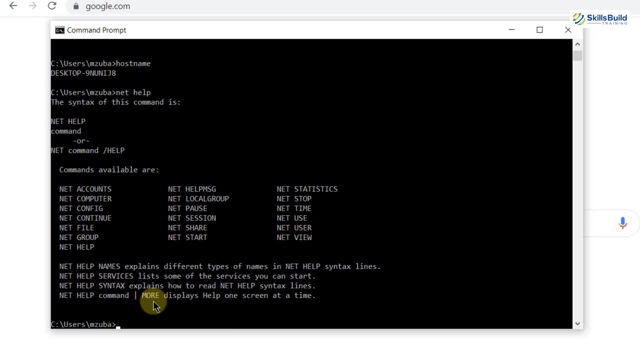 i will just write net help x, c, system ls, which will give me the information about open In NET, and i will have a lot of information about that one. so just hit enter and these are the commands which are available with respect to the net command. so if i write here only net, again i have this information. 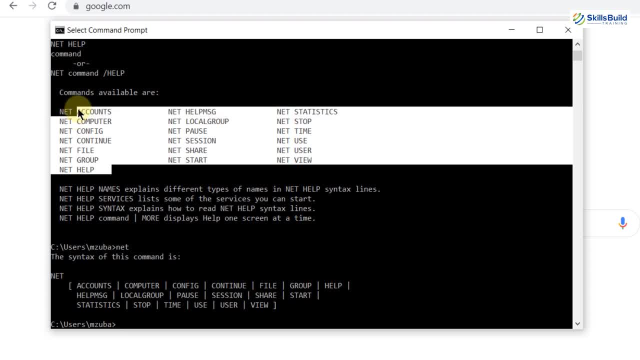 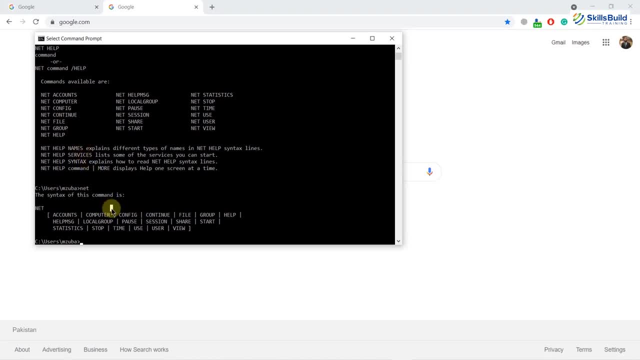 so what i can do. i can use a net command with the addition of these commands and i'll be able to get a lot of information. and that brings us to the end of this video. i hope you enjoyed watching this video. please leave a like and subscribe to our. 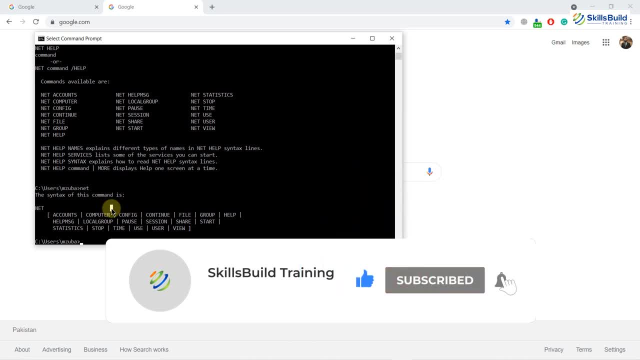 channel, as this channel is all about showing you how to become an it pro really fast. if you have something to ask, please leave a comment below. we will get back to you as soon as possible. we will see you in another video. till then, take care.